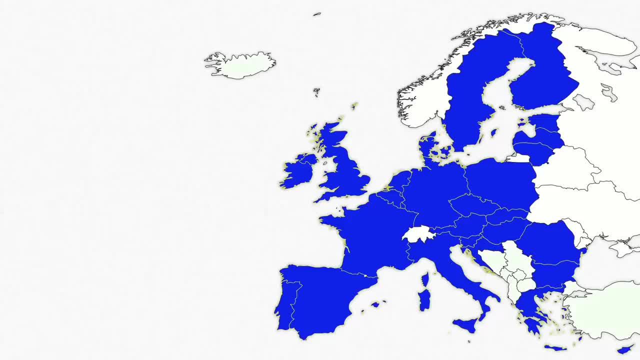 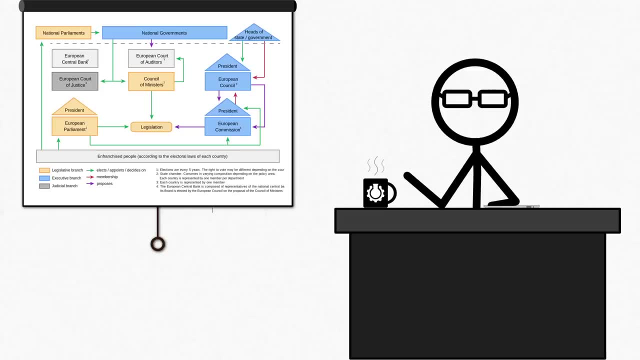 Luxembourg and Malta. The edges of the EU will probably continue to expand further out, as there are other countries in various stages of trying to become a member. How the EU works is hideously complicated and a story for another time, but for this video. 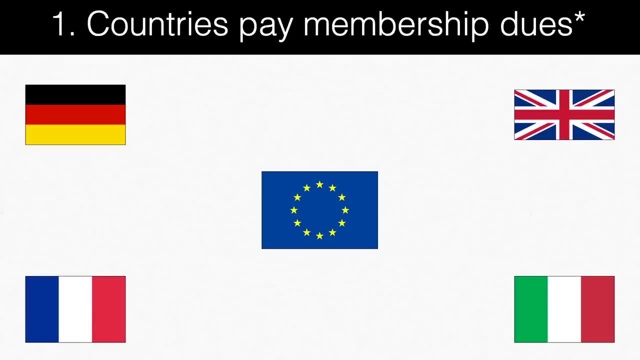 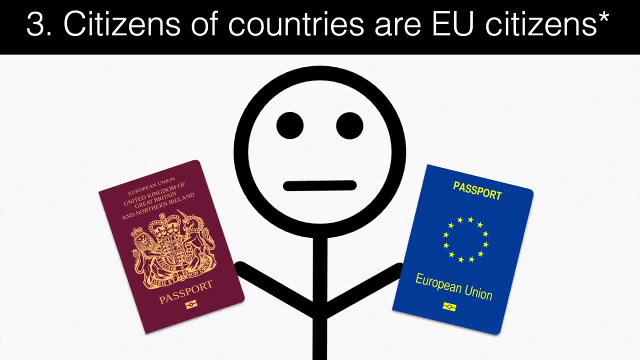 you need know only three things: First, countries pay membership dues and second vote on the laws they all must follow. and third, citizens of member countries are automatically European Union citizens as well. This last means that if you are a citizen of any of these, 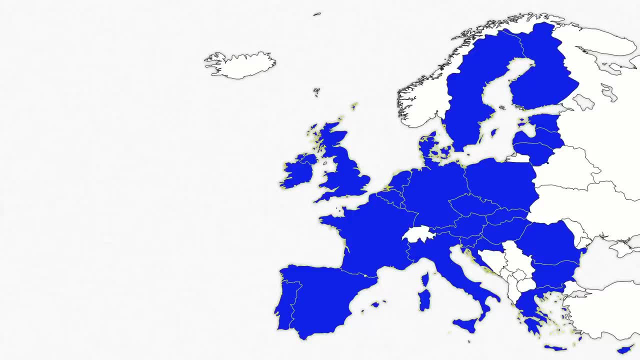 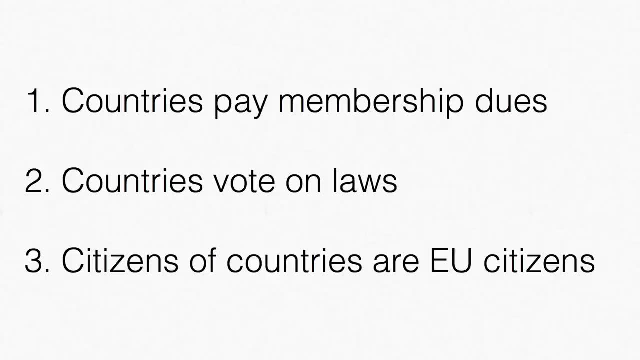 countries. you are free to live and work and retire in any of the others, which is nice, especially if you think your country is too big or too small, or too hot or too cold. The European Union gives you options. By the way, did you notice how all three of these statements have? 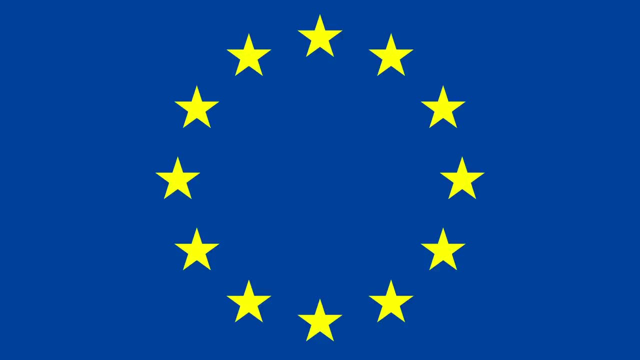 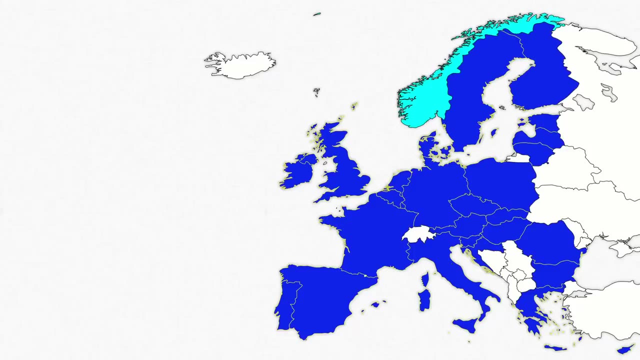 asterisks attached to this unhelpful footnote. Well, get used to it. Europe loves asterisks that add exceptions to complicated agreements. These three, for example, point us towards the first bit of border fuzziness with Norway, Iceland and Little Liechtenstein. none of 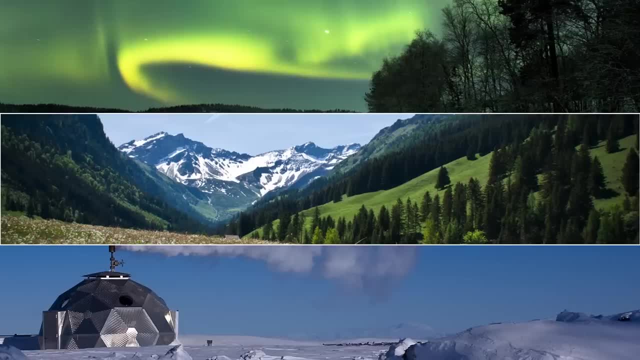 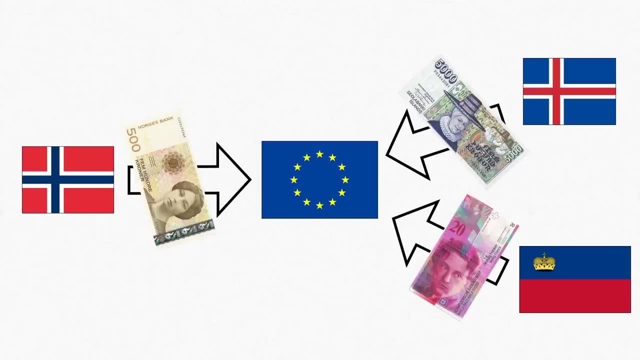 which are in the European Union, but if you're an EU citizen, you can live in these countries, and Norwegians, Icelanders or Liechtensteiners can live in yours. Why, In exchange for freedom of movement of people, they have to pay membership fees to the European Union, even though they 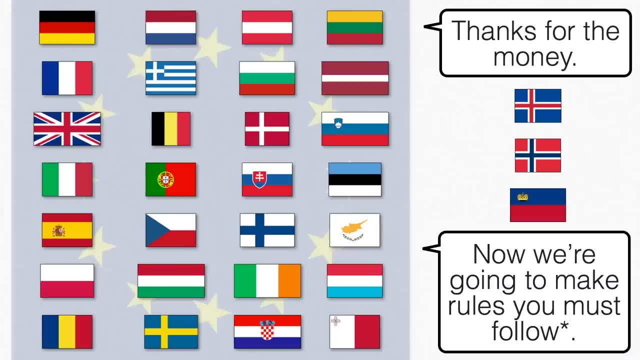 aren't a part of it and thus don't get a say in its laws that they still have to follow. This arrangement is the European Economic Area, and it sounds like a terrible deal, were it not for that asterisk, which grants EEA, but not EU members, a pass on some areas of law, notably 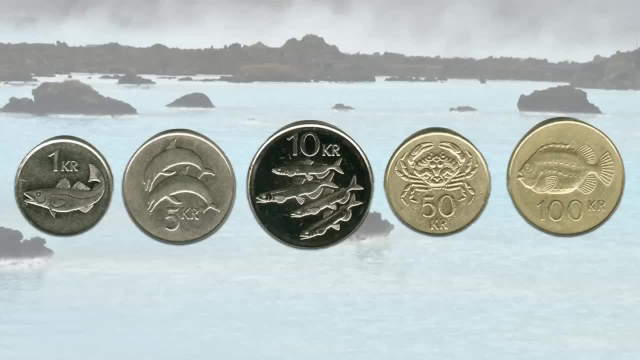 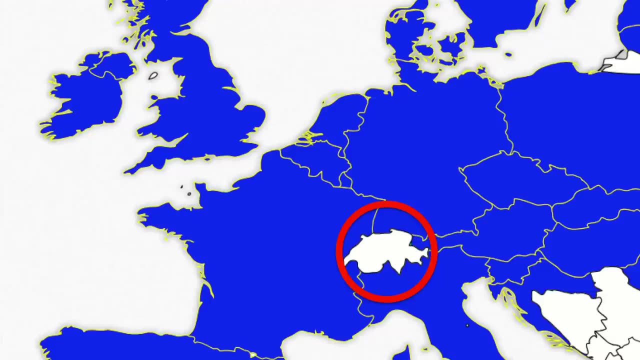 farming and fishing, something a country like, say, Iceland might care quite a lot about. running themselves Between the European Union and the European Economic Area, the continent looks mostly covered, with the notable exception of Switzerland, who remains neutral and fiercely independent, except for her participation in the Schengen Area. If you're from a country, 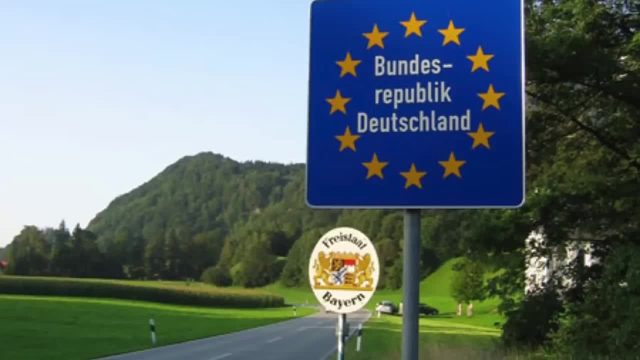 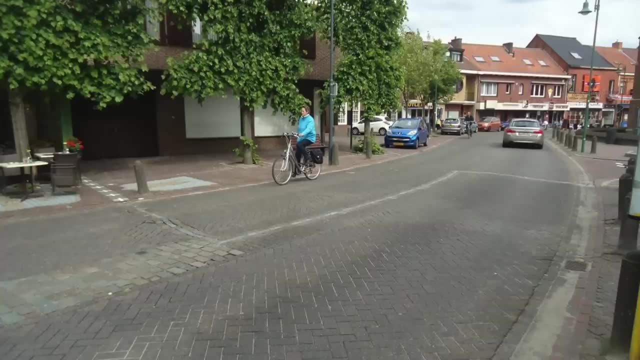 that keeps her borders extremely clean and or well-patrolled. the Schengen Area is a bit mind-blowing because it's an agreement between countries to take a meh approach to borders In the Schengen Area. international boundaries look like this: No border officers or passport. 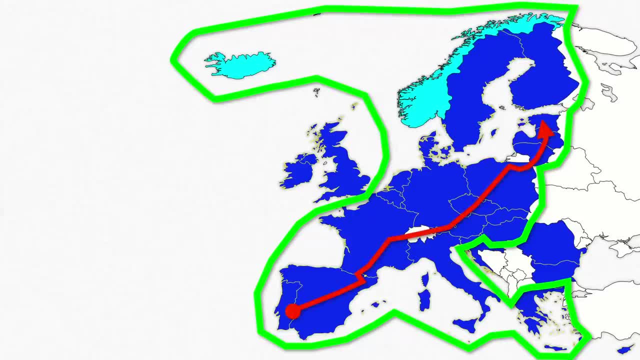 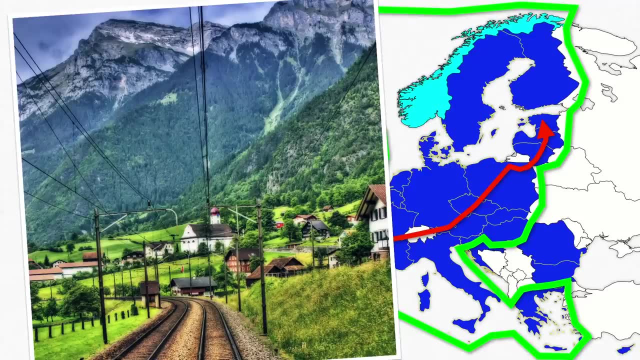 checks of any kind. You can walk from Lisbon to Tallinn without identification or the need to answer the question business or pleasure. For Switzerland, being part of Schengen but not part of the European Union means that non-Swiss can check in any time they like. 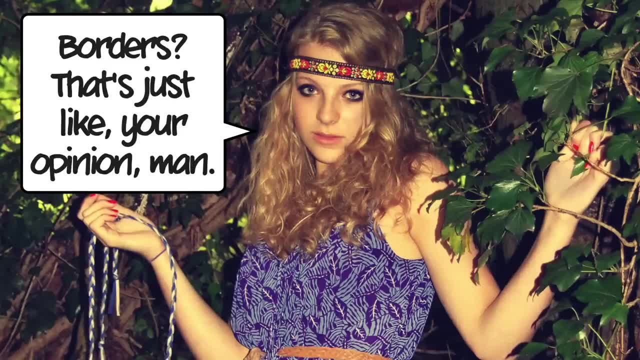 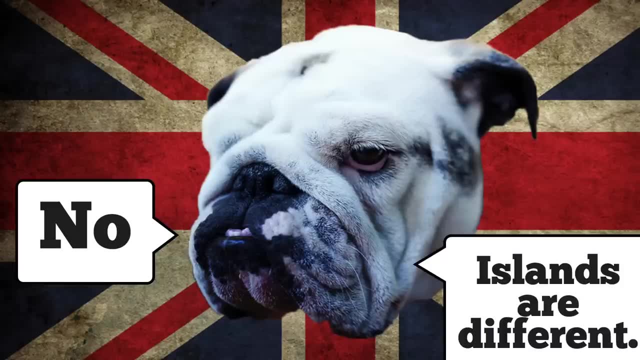 but they can never stay. This kumbaya approach to borders isn't appreciated by everyone in the EU, Most loudly the United Kingdom and Ireland, who argue that islands are different. Thus, to get onto these fair isles, you'll need a passport and a good reason. 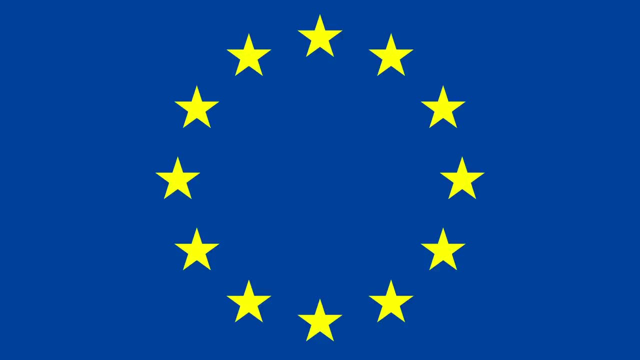 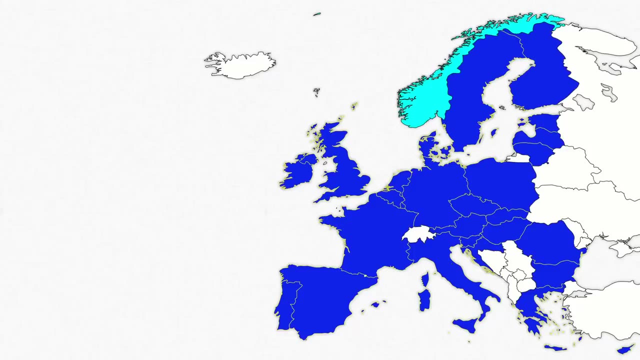 asterisks attached to this unhelpful footnote. Well, get used to it. Europe loves asterisks that add exceptions to complicated agreements. These three, for example, point us towards the first bit of border fuzziness with Norway, Iceland and Little Liechtenstein. none of 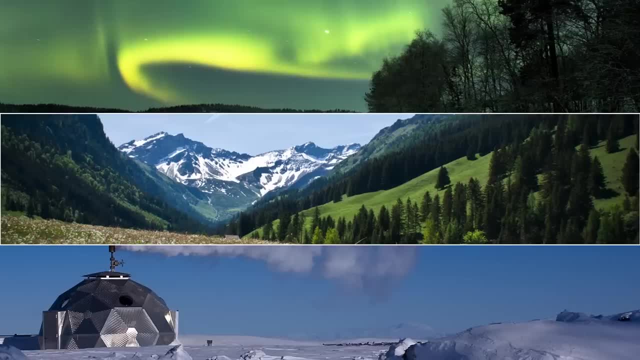 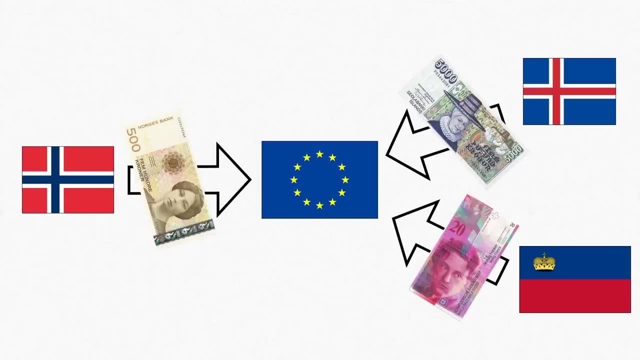 which are in the European Union, but if you're an EU citizen, you can live in these countries, and Norwegians, Icelanders or Liechtensteiners can live in yours. Why, In exchange for freedom of movement of people, they have to pay membership fees to the European Union, even though they 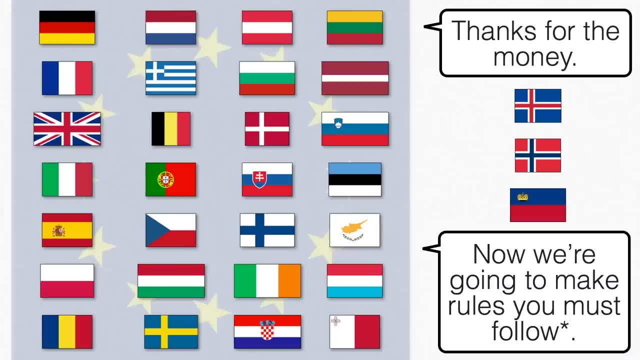 aren't a part of it and thus don't get a say in its laws that they still have to follow. This arrangement is the European Economic Area, and it sounds like a terrible deal, were it not for that asterisk, which grants EEA, but not EU members, a pass on some areas of law, notably 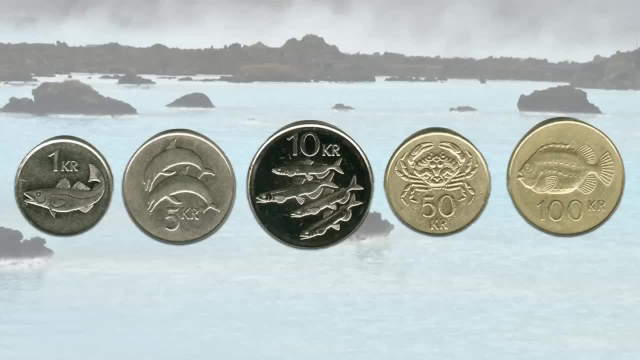 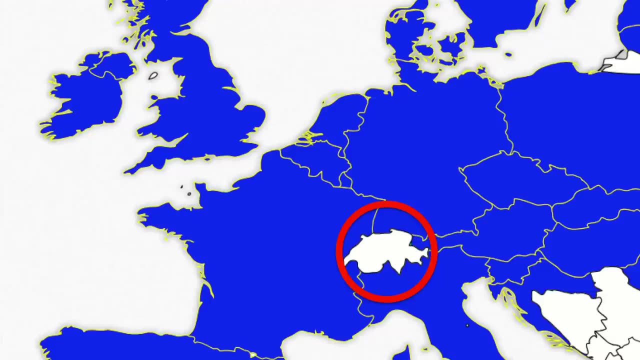 farming and fishing, something a country like, say, Iceland might care quite a lot about. running themselves Between the European Union and the European Economic Area, the continent looks mostly covered, with the notable exception of Switzerland, who remains neutral and fiercely independent, except for her participation in the Schengen Area. If you're from a country, 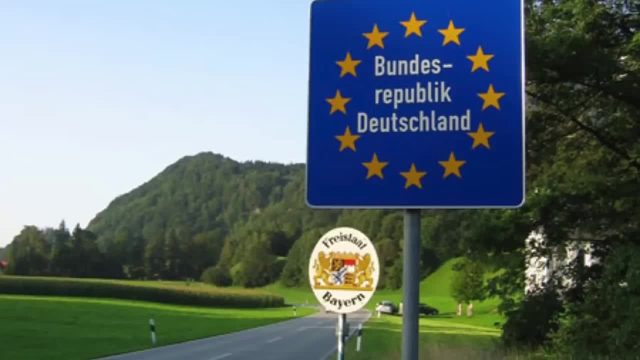 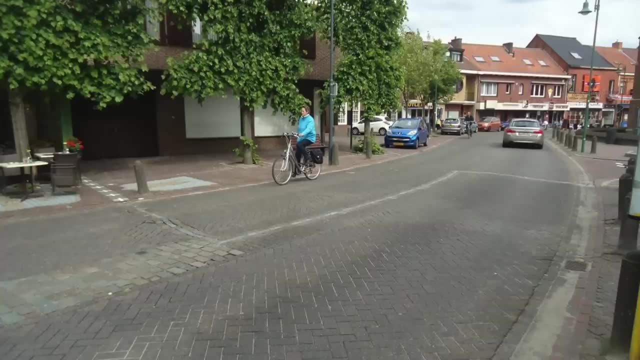 that keeps her borders extremely clean and or well-patrolled. the Schengen Area is a bit mind-blowing because it's an agreement between countries to take a meh approach to borders In the Schengen Area. international boundaries look like this: No border officers or passport. 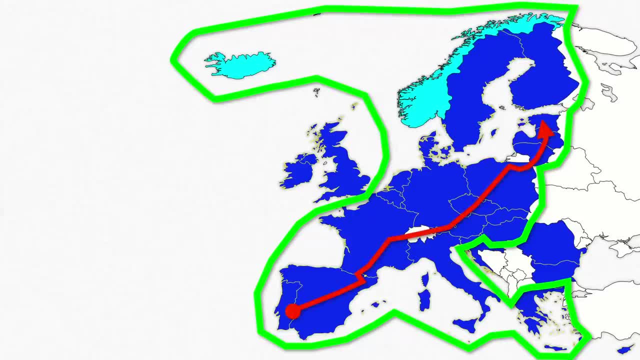 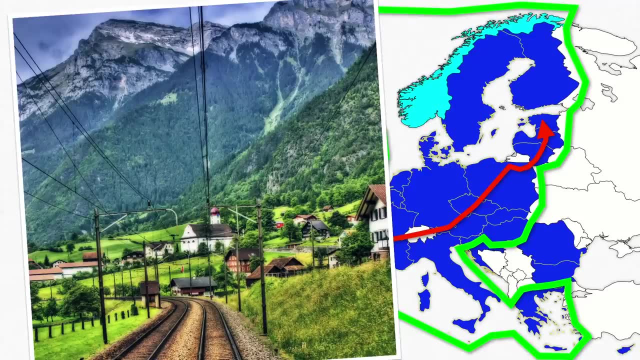 checks of any kind. You can walk from Lisbon to Tallinn without identification or the need to answer the question business or pleasure. For Switzerland, being part of Schengen but not part of the European Union means that non-Swiss can check in any time they like. 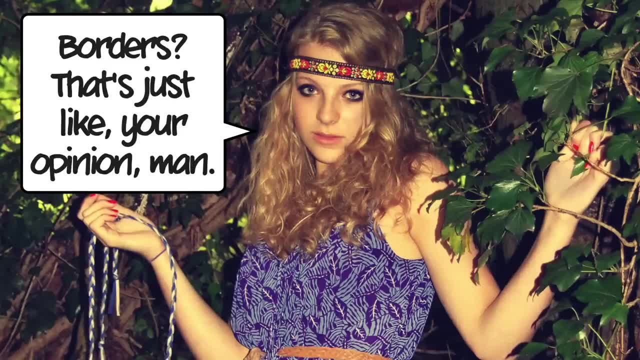 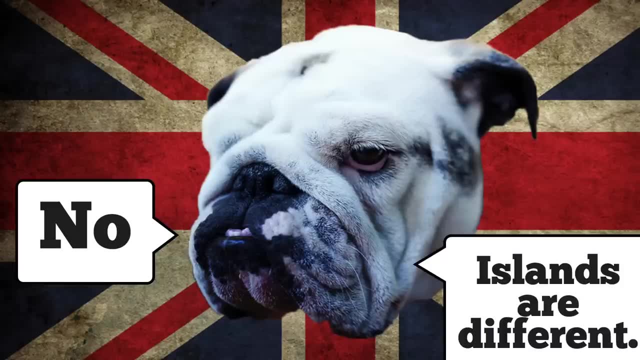 but they can never stay. This kumbaya approach to borders isn't appreciated by everyone in the EU, Most loudly the United Kingdom and Ireland, who argue that islands are different. Thus, to get onto these fair isles, you'll need a passport and a good reason. 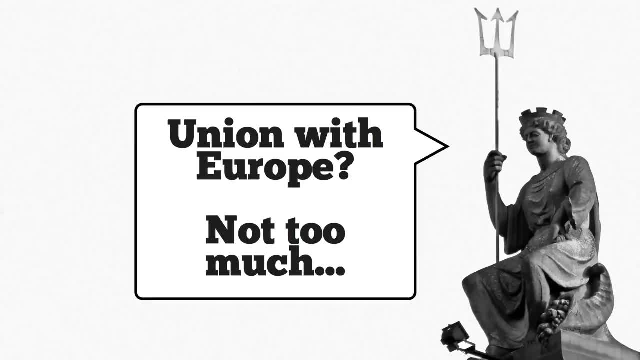 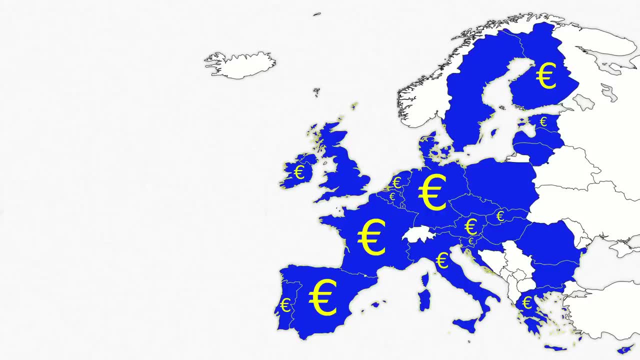 Britannia's reluctance to get fully involved with the EU brings us to the next topic: money. The European Union has its own fancy currency, the Euro, used by the majority but not all of the European Union members. This economic union is called the Eurozone. 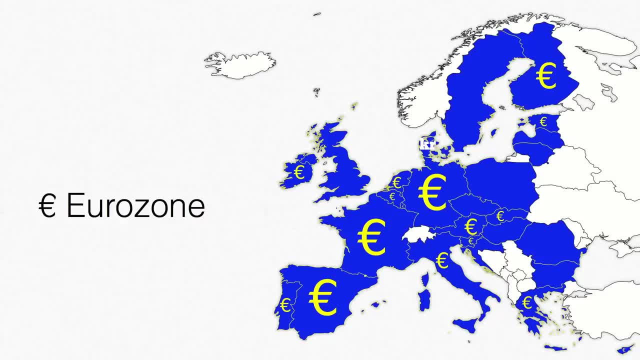 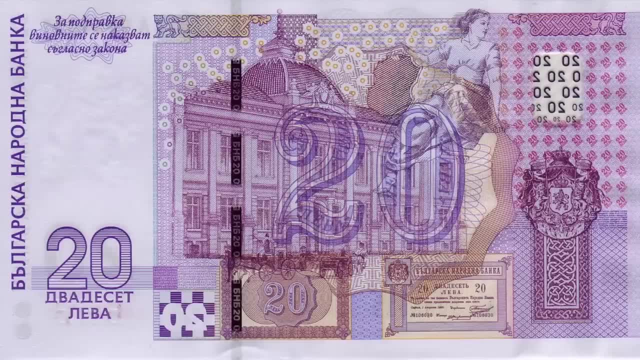 and to join a country must first reach certain financial goals, And lying about reaching those goals is certainly not something anyone would do. Most of the Eurozone members, when they meet the goals, will ditch their local currency in favor of the Euro. 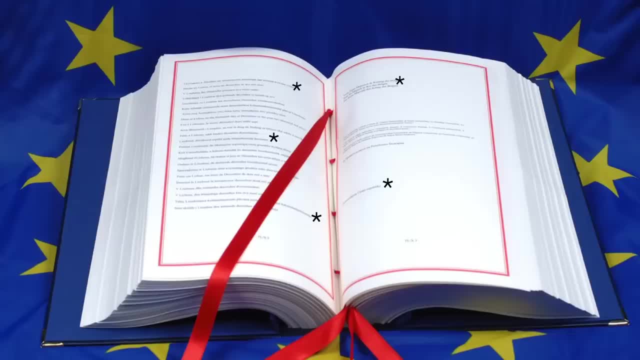 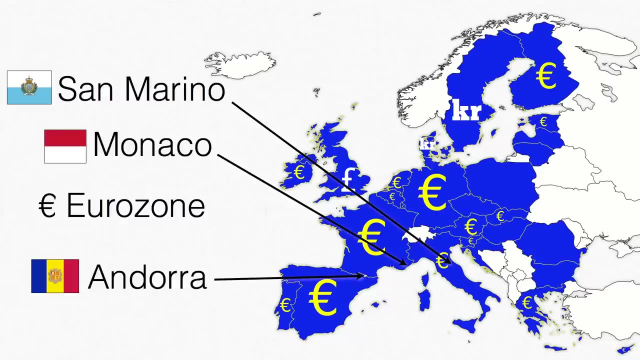 but three of them- Denmark, Sweden and, of course, the United Kingdom- have asterisks attached to the Euro section of the treaty, giving them a permanent opt-out. And, weirdly, four tiny European countries- Andorra, San Marino, Monaco and Vatican City- have an asterisk giving. 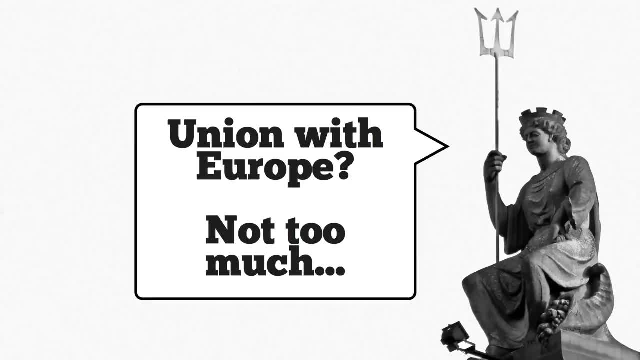 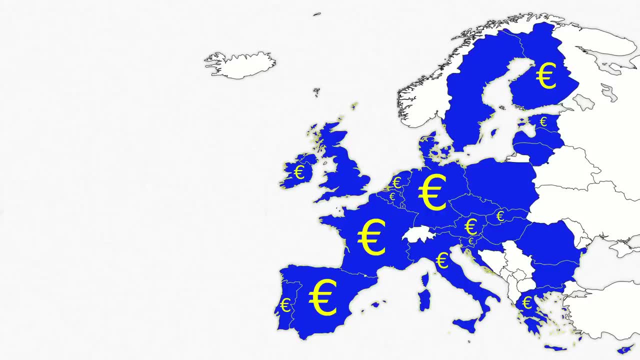 Britannia's reluctance to get fully involved with the EU brings us to the next topic: money. The European Union has its own fancy currency, the Euro, used by the majority but not all of the European Union members. This economic union is called the Eurozone. 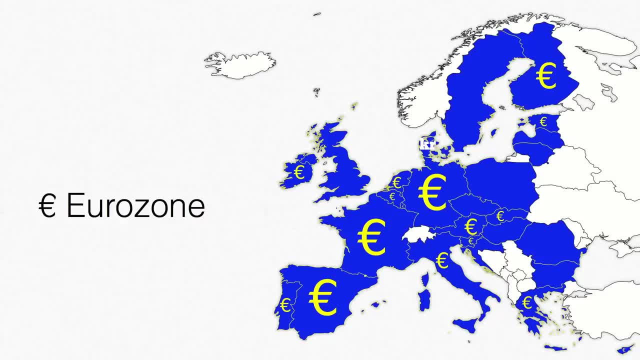 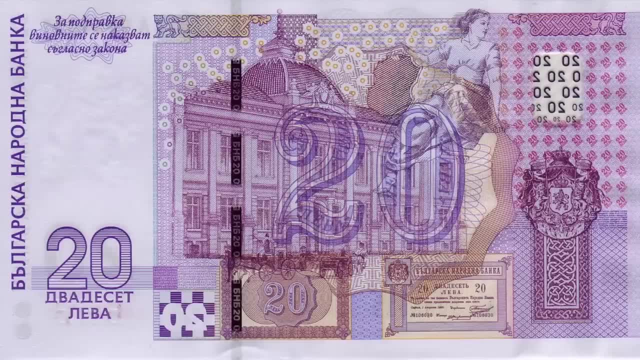 and to join a country must first reach certain financial goals, And lying about reaching those goals is certainly not something anyone would do. Most of the Eurozone members, when they meet the goals, will ditch their local currency in favor of the Euro. 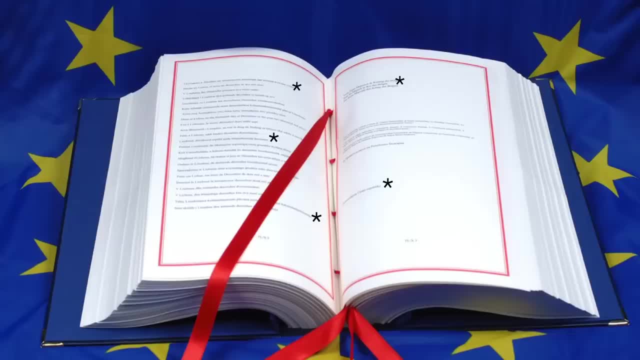 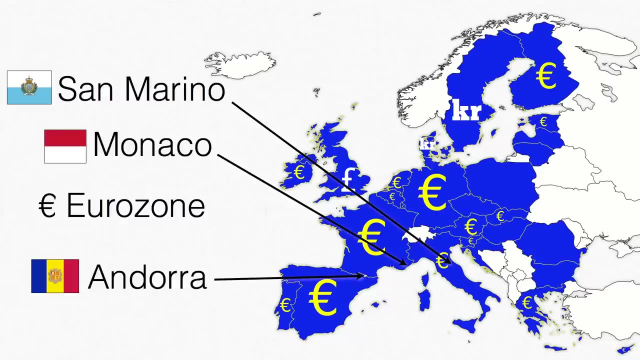 but three of them- Denmark, Sweden and, of course, the United Kingdom- have asterisks attached to the Euro section of the treaty, giving them a permanent opt-out. And, weirdly, four tiny European countries- Andorra, San Marino, Monaco and Vatican City- have an asterisk giving. 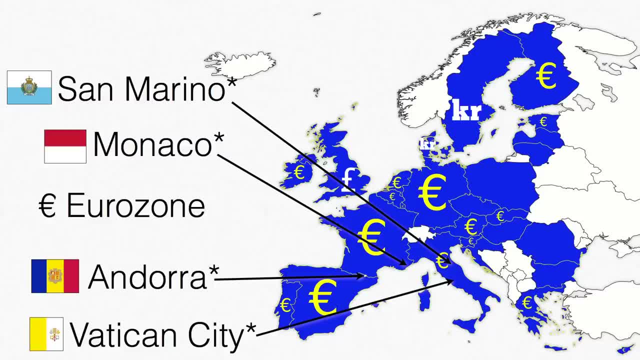 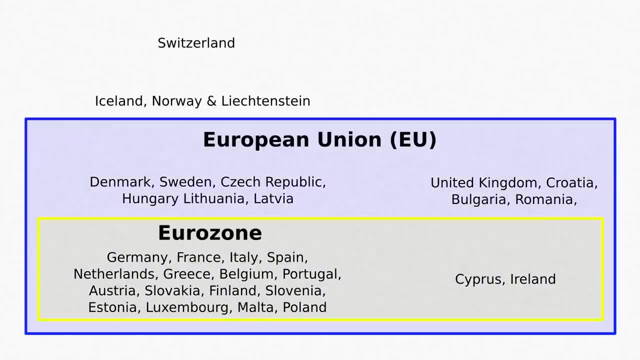 them the exact reverse: the right to print and use Euros as their money despite not being in the European Union at all. So that's the big picture. There's the EU which makes all the rules, the Eurozone inside of it, with a common currency. the European Economic Area outside. 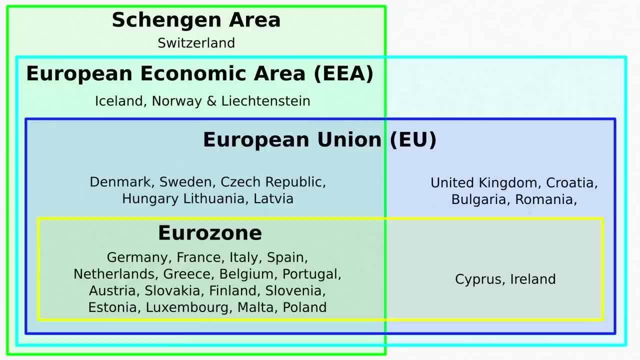 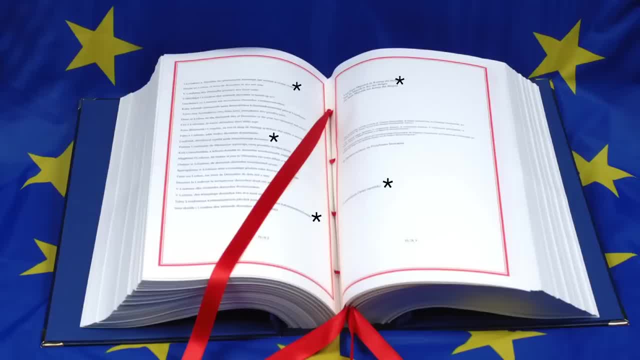 where people can move freely, and the selective Schengen for countries that think borders just aren't worth the hassle. As you can see, there's some strange overlap with these borders, but we're not done talking about complications by a long shot. Once again, because empire. So Portugal and Spain have islands from their colonial days that they've never parted with. These are the Madeira and Canary Islands, off the coast of Africa, and the Azores, well into the Atlantic. Because these islands are Spanish and Portuguese, they're part of the European Union. 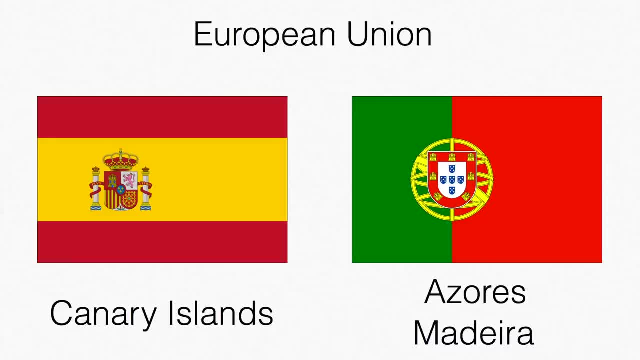 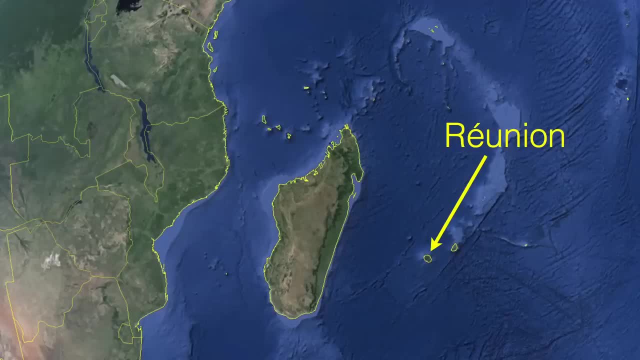 as well. Adding a few islands to the EU's borders isn't a big deal, until you consider France, the queen of not letting go. She still holds on to a bunch of islands in the Caribbean: Reunion off the coast of Madagascar, and French Guiana in South America. As far as France is, 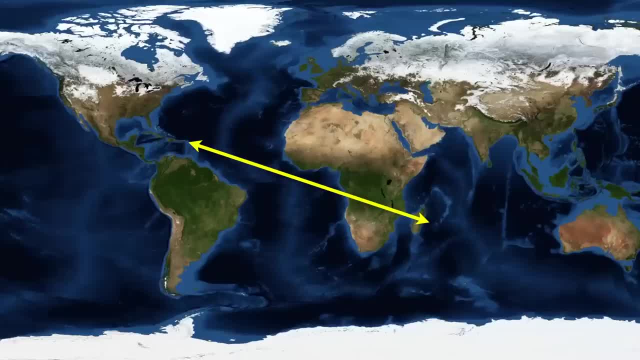 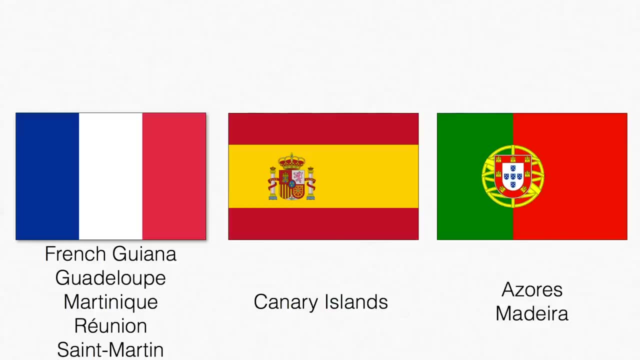 concerned. these are France too, which single-handedly extends the edge-to-edge distance of the European Union across a third of the Earth's circumference. Collectively, these bits of France, Spain and Portugal are called the outermost regions, and they're the 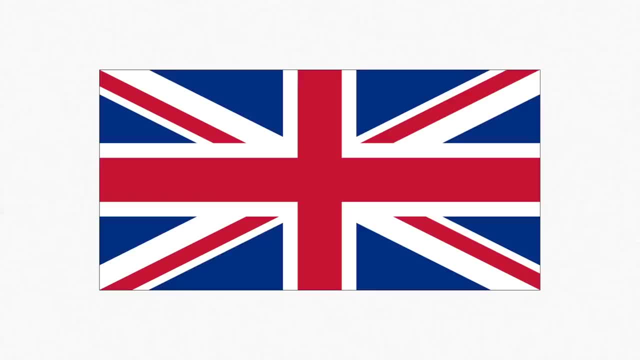 result of the simple answer to empire: just keep it. On the other hand, there's the United Kingdom, the master of maintaining complicated relationships with her quasi-former land. The United Kingdom, the master of maintaining complicated relationships with her quasi-former land. 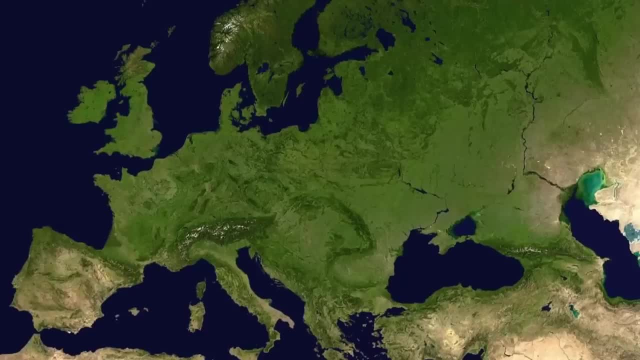 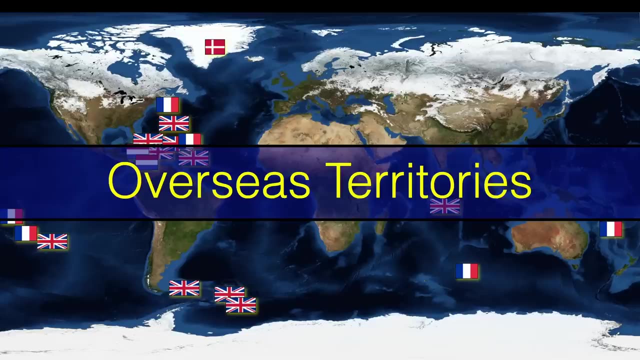 And she's by no means alone in this on such an empire-happy continent. The Netherlands and Denmark and France again all have what the European Union calls overseas territories. They're not part of the European Union. instead, they're a bottomless well of asterisks due to. 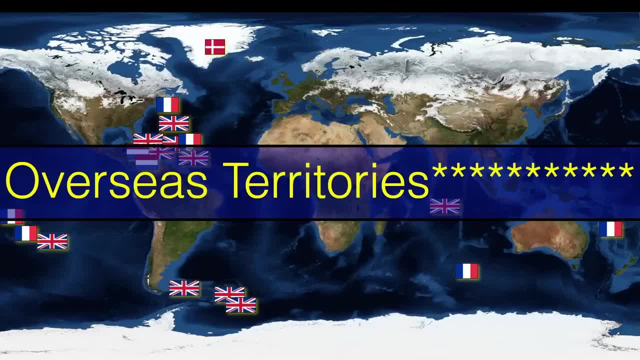 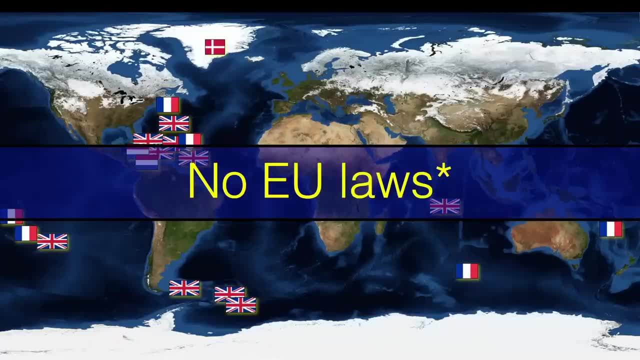 their complicated relationships with both the European Union and their associated countries, Which makes it hard to say anything meaningful about them as a group. but In general, European Union law doesn't apply to these places, though in general, the people who live there are European Union citizens, because, in general, 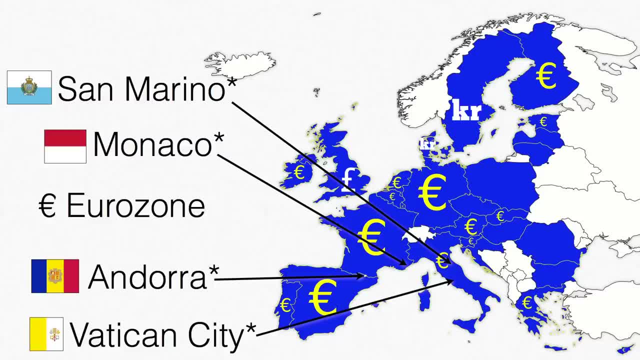 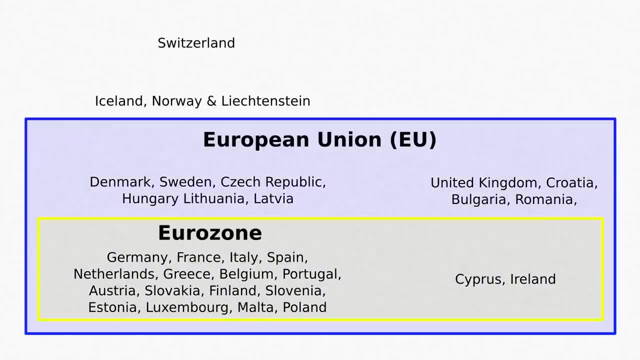 them the exact reverse: the right to print and use Euros as their money despite not being in the European Union at all. So that's the big picture. There's the EU which makes all the rules, the Eurozone inside of it, with a common currency. the European Economic Area outside. 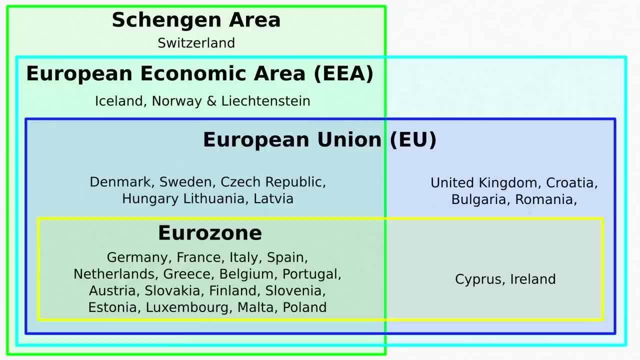 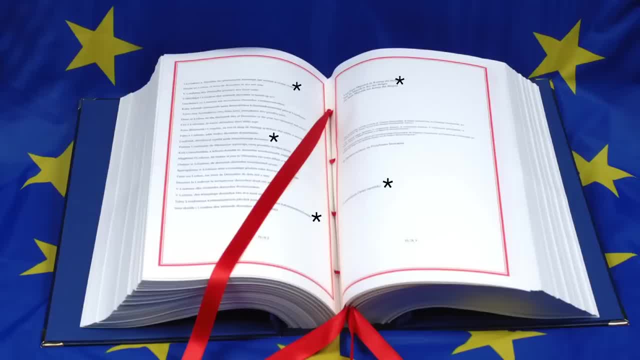 where people can move freely, and the selective Schengen for countries that think borders just aren't worth the hassle. As you can see, there's some strange overlap with these borders, but we're not done talking about complications by a long shot. Once again, because empire. 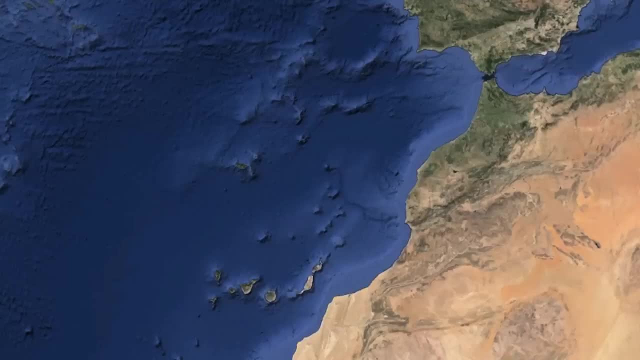 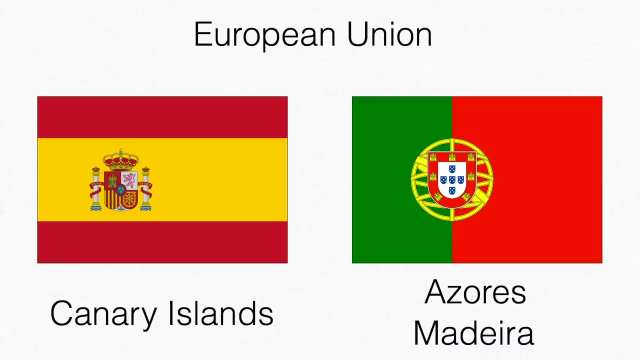 So Portugal and Spain have islands from their colonial days that they've never parted with. These are the Madeira and Canary Islands, off the coast of Africa, and the Azores, well into the Atlantic. Because these islands are Spanish and Portuguese, they're part of the European Union. 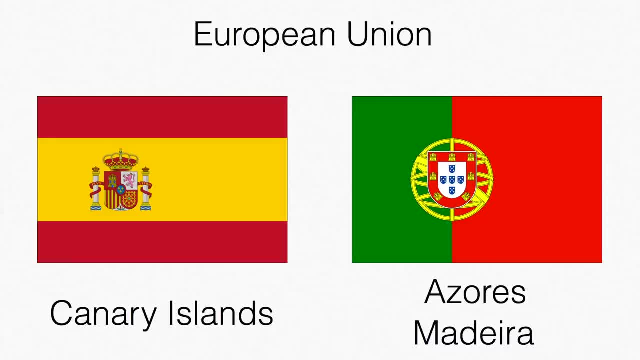 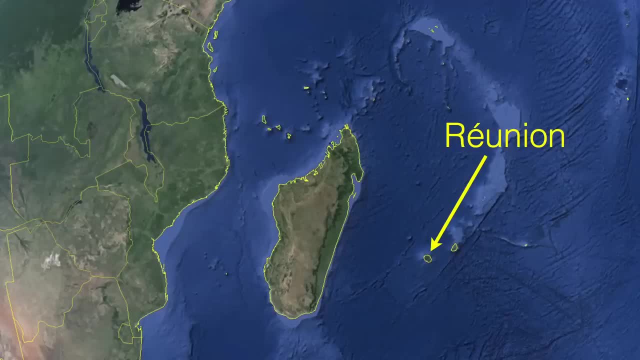 as well. Adding a few islands to the EU's borders isn't a big deal, until you consider France, the queen of not letting go. She still holds on to a bunch of islands in the Caribbean: Reunion off the coast of Madagascar, and French Guiana in South America. As far as France is, 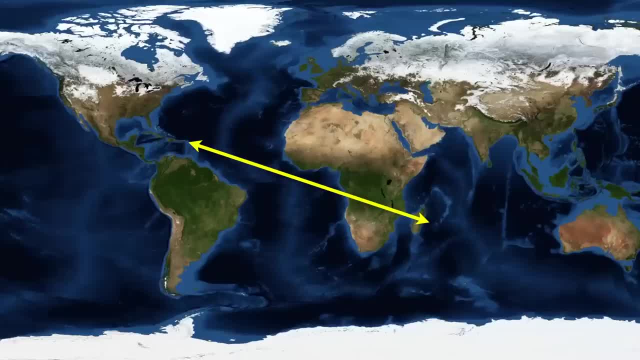 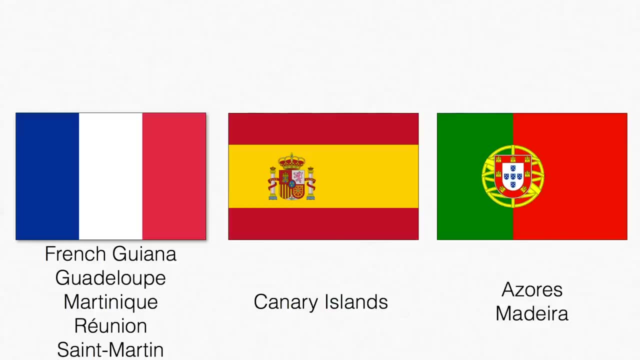 concerned. these are France too, which single-handedly extends the edge-to-edge distance of the European Union across a third of the Earth's circumference. Collectively, these bits of France, Spain and Portugal are called the outermost regions, and they're the 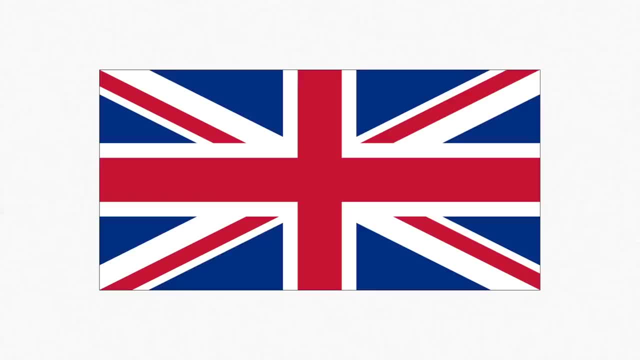 result of the simple answer to empire: just keep it. On the other hand, there's the United Kingdom, the master of maintaining complicated relationships with her quasi-former land. The United Kingdom, the master of maintaining complicated relationships with her quasi-former land. 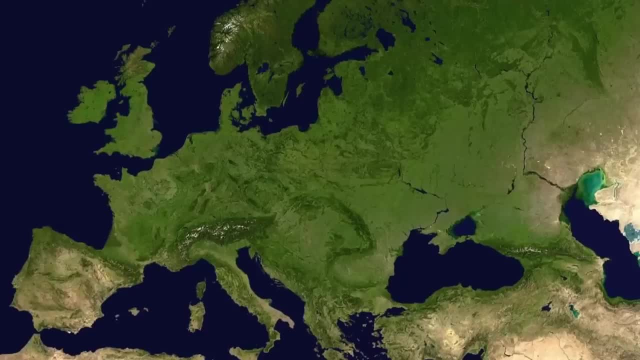 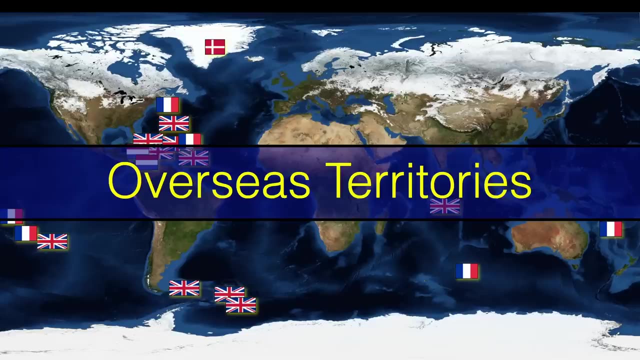 And she's by no means alone in this on such an empire-happy continent. The Netherlands and Denmark and France again all have what the European Union calls overseas territories. They're not part of the European Union. instead, they're a bottomless well of asterisks due to. 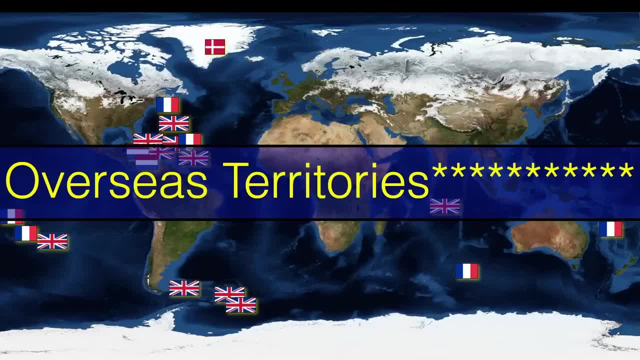 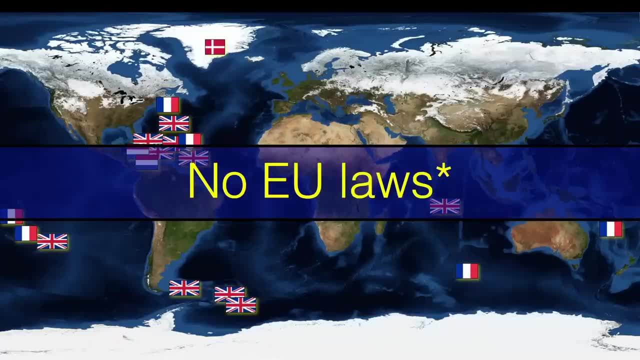 their complicated relationships with both the European Union and their associated countries, Which makes it hard to say anything meaningful about them as a group. but In general, European Union law doesn't apply to these places, though in general, the people who live there are European Union citizens, because, in general, 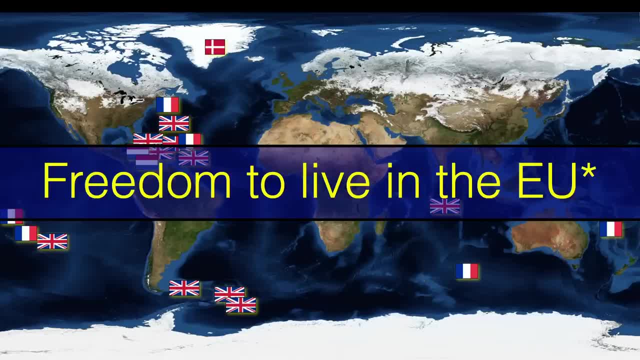 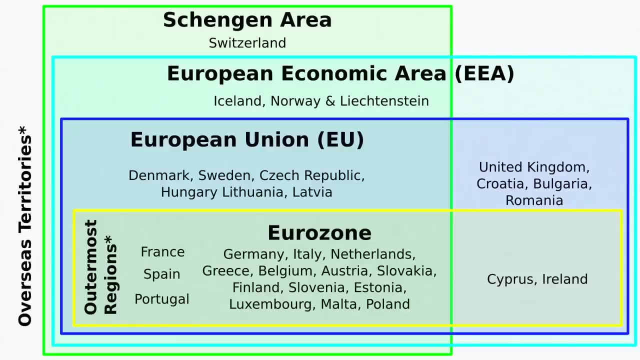 they have the citizenship of their associated country, so in general they can live anywhere in the EU they want. but in general other European Union citizens can't freely move to these territories, Which makes these places a weird semi-permeable membrane of the European Union. 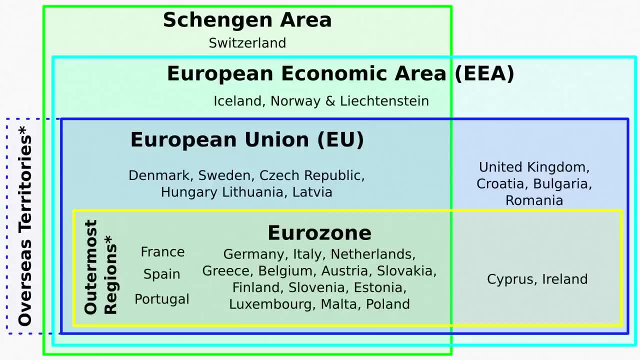 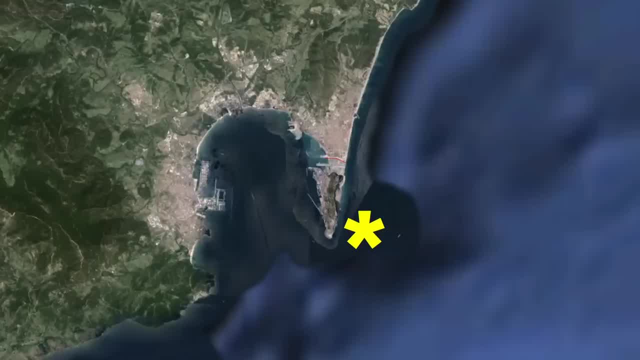 proper and the final part we're going to talk about in detail, even though there are still many more one-off asterisks you might stumble upon, such as the Isle of Man, or those Spanish cities in North Africa, or Gibraltar, who pretends to be part of Southwest England sometimes, or that.